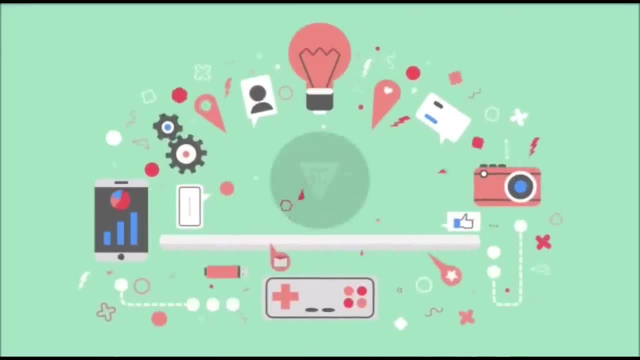 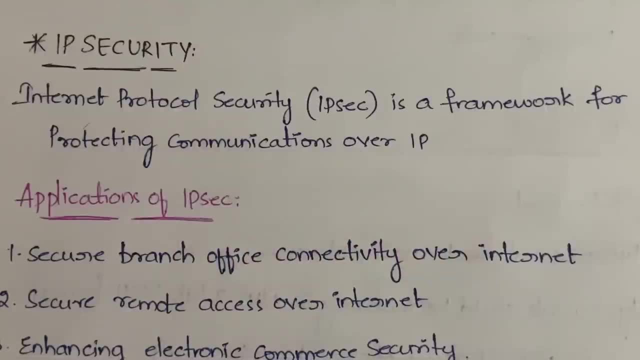 Hello everyone, welcome back to my YouTube channel: travel free. In this video, I am going to explain you about IP security in the subject of cryptography and network security. So basically, in this video I will explain you what is IP security and the applications of IP security, and also the architecture of IP security. 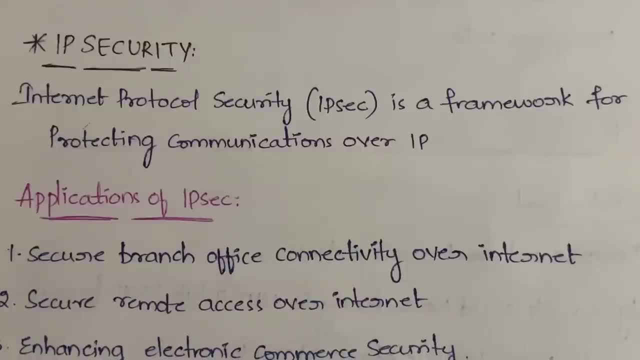 Okay, and we will have different, different components in the architecture. about those things we will be discussing in a separate videos. Okay, so for this video: what is IP security, What are the applications of IP security and what is the architecture of IP security? Okay, so let's get into the video now. And before that I also started a new channel with study abroad content. If you are having interest, then I will give you the link of the channel in the description. You can have a look. Now let us get into the video First. IP security is nothing but internet protocol. 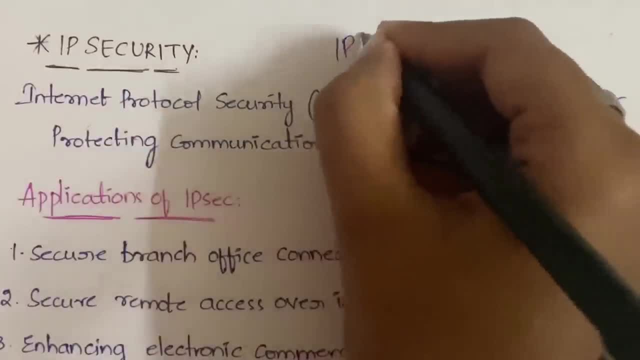 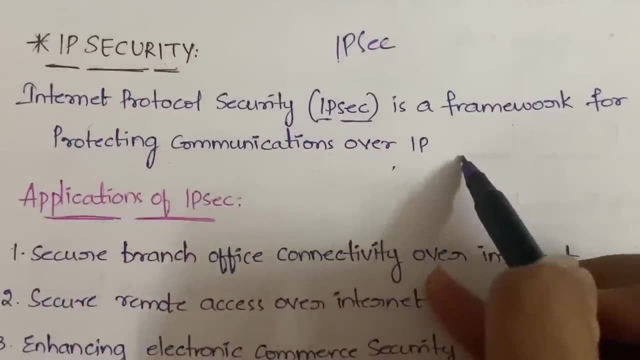 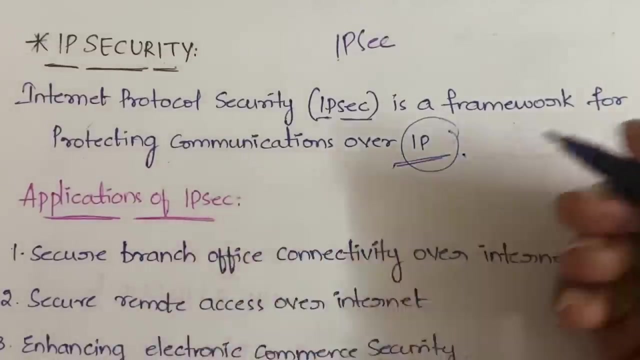 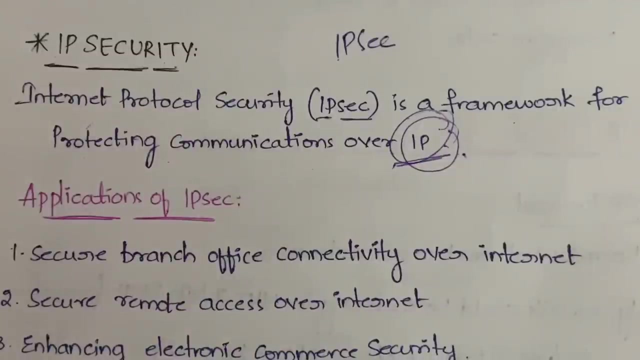 Security. Okay, that is, in short, also called as IP SEC. Okay, IP security. Okay, it is a framework for protecting communications over IP, that is, with the help of internet protocol, you will be doing communications right. It could be email, or it could be any simple text or anything. By using the internet protocol, you are communicating Right. So in order to protect those communications, in order to establish security for those kind of communications, we will be using 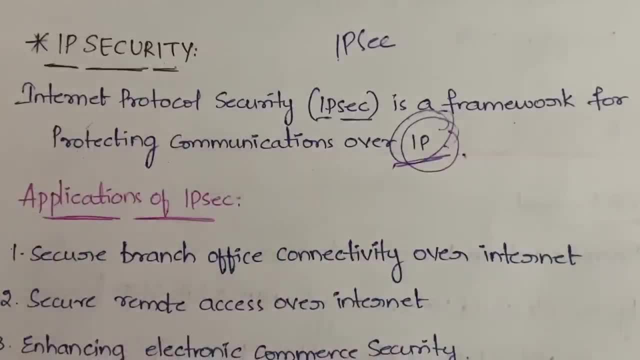 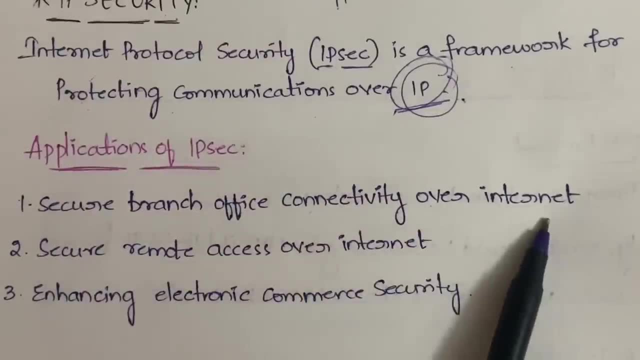 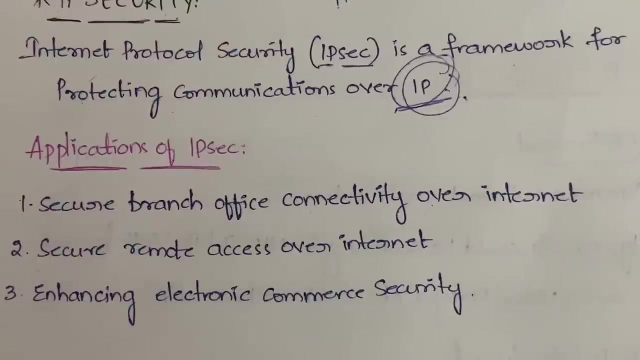 this IP security. Okay, so what are the applications of IP security? Let us see now. First is secure branch office connectivity over internet. that is secure branch, like you will be, you can say like inter branch connectivity, one branch to other branch. suppose we let us take a bank, So bank will have different, different branches, right? So each and every branch has to be connected with each other And bank is something which is very confidential, So it needs some security. 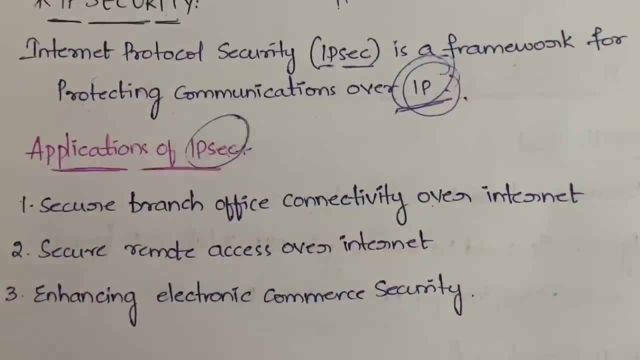 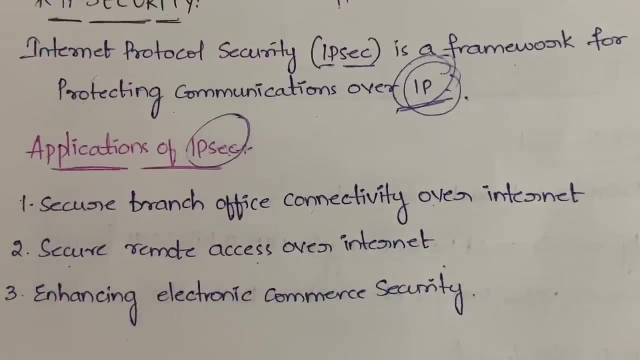 So in that case, you will be using this IP security, Okay, and secure remote access over internet. See, nowadays everybody is doing work from home, right? So everybody needs remote desktop because they are working from home, they need some remote desktop through which they can work from their home as well. But when you are working with remote desktop on your personal computer- which is something again risky, right, Because remote desktop belongs to your computer- 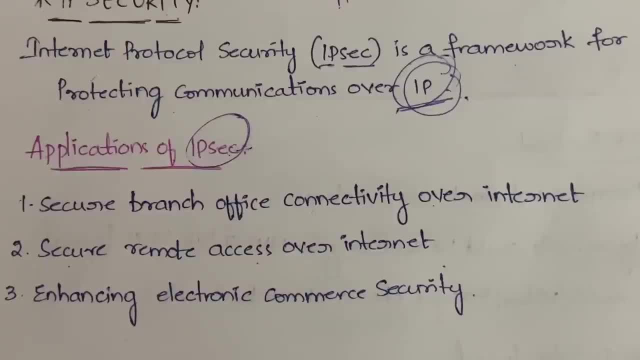 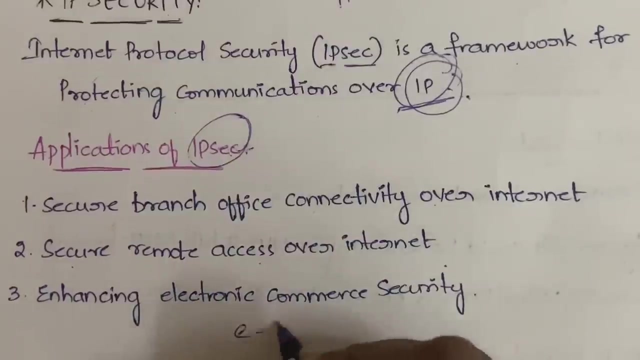 to your company or it belongs to a particular client, so you are bringing their data onto your personal computer. then in that case also, you need some security. that is also provided by ipsec and enhancing electronic commerce security. you know what is electronic commerce, e-commerce- so you're. 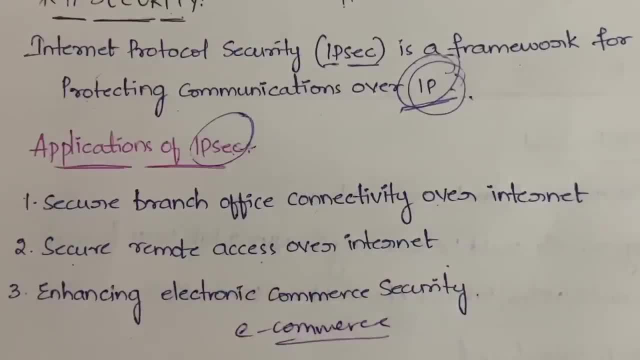 buying some sites. sorry, sorry, not sites. you're buying some uh products from the e-commerce sites like amazon or flipkart and you will be doing the payment as well, right? so the payment has to securely reach from your bank account to the amazon bank account. in between, it has to not go. 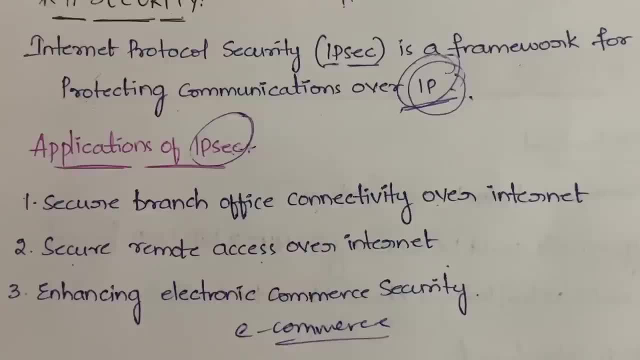 into anybody's bank account, and if you are requesting for a refund, it has to securely come from amazon to your bank account, so that also needs security. in that case also, you'll be using this ipsec. not only this. if you know any other examples, you can write where you are using internet. 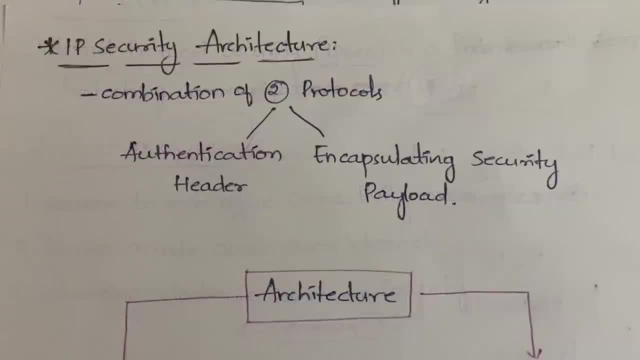 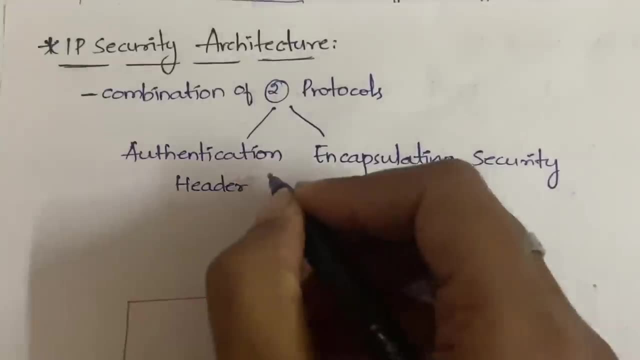 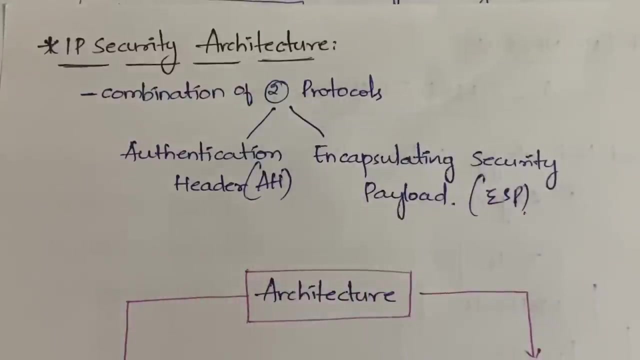 protocol security. okay, so now let us see the architecture of ip. so if you look at the architecture of ip security, it is a combination of two protocols, okay. first one is authentication header, which is also ah, and the second one is encapsulating security payload, esp. okay, so to a combination of two. 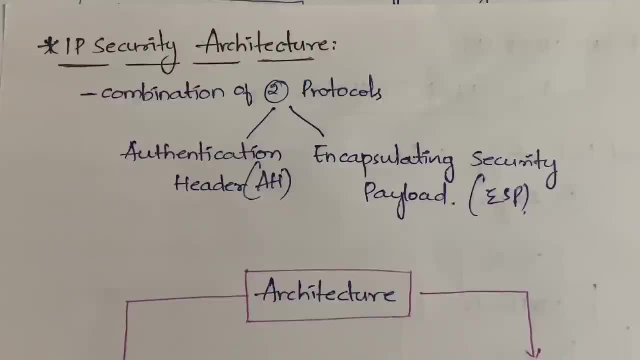 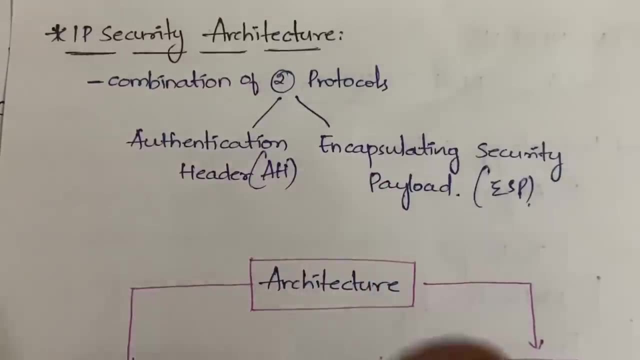 protocols: authentication header, encapsulation payload. so about authentication header- i will be explaining in a separate video- and encapsulating security payload, also separate or otherwise. i'll try to mix up these two things. okay, let us see according to the length of the video, i'll do it. 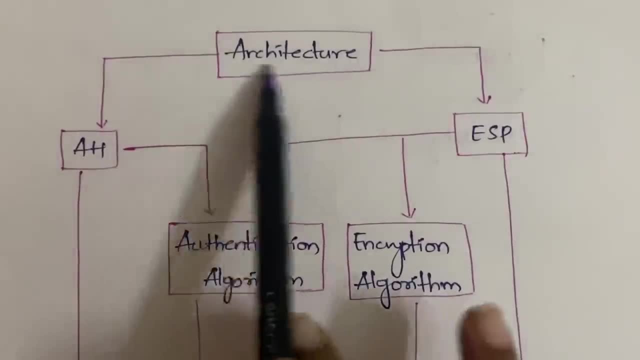 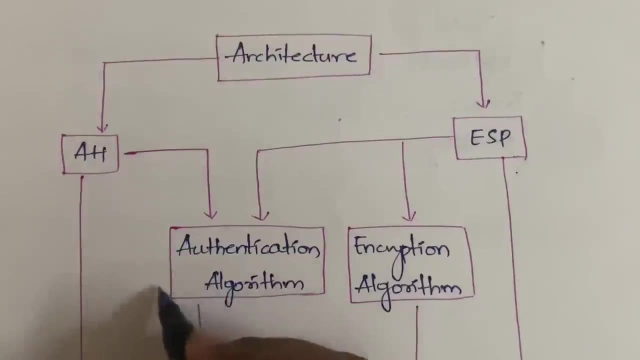 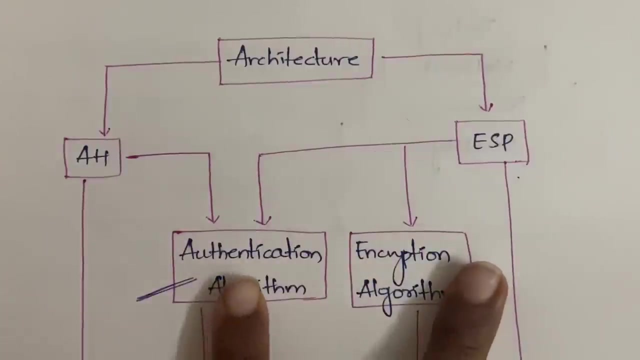 so now let us see the architecture. so this is the architecture: two protocols: authentication header and encapsulating security payload. so authentication header is responsible for the authentication, okay, and by using encapsulating security payload, you can get both authentication and encryption. got it: by this you get only authentication, whereas by esp, encapsulating security payload, you can get both authentication.